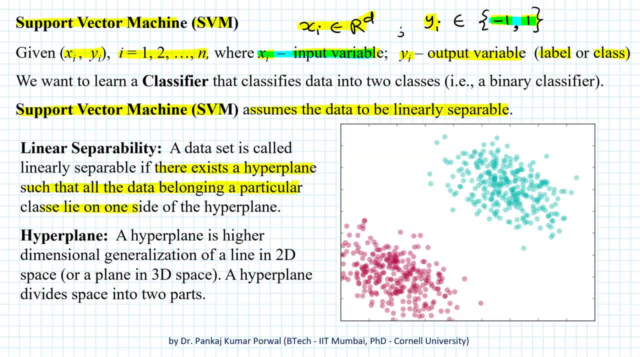 belonging to a particular class lie on one side of the hyperplane, and a hyperplane is nothing but higher dimensional generalization of what is a line in 2D or a plane in 2D, A plane in 3D, and a hyperplane basically divides space into two parts, For example, the two 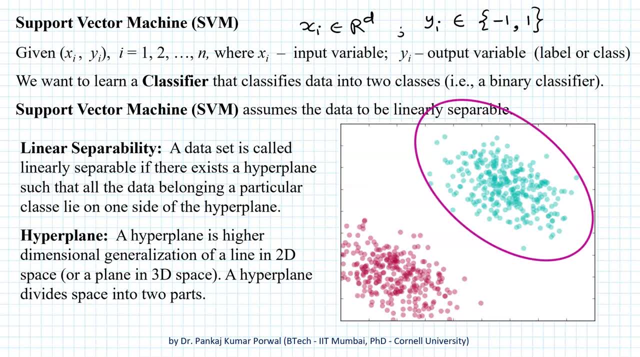 dimensional data consisting of blue dots and pink dots shown in the figure is linearly separable because I can draw a line such that all the data belonging to a particular class lies on the one side of the hyperplane. So, for example, here the blue data lies on the 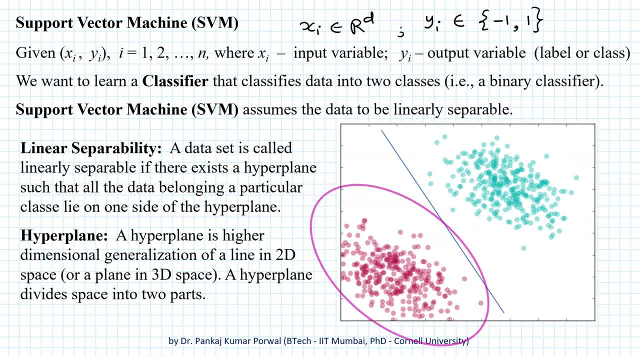 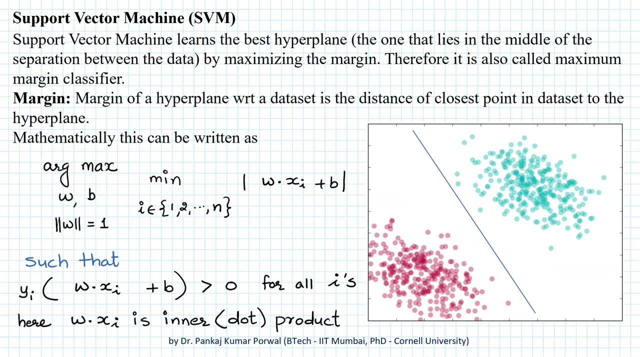 right side of the line and the pink data. However, if our data is linearly separable, then there will be infinitely many such lines or hyperplanes that will partition our data. So which of the hyperplane should we select And support? vector machine helps us identify the best hyperplane, that is the one that lies. 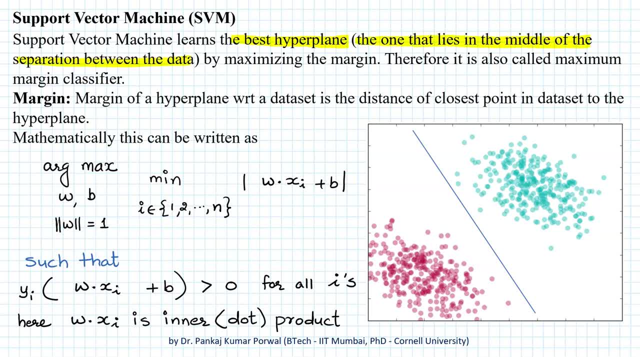 in the middle of the separation between the data By maximizing the margin. that is why it is also called maximum margin classifier. So now, what is the margin? the margin of the hyperplane is nothing but the distance of the closest point in the data set to the hyperplane. So, for example, here, if I look at this hyperplane, 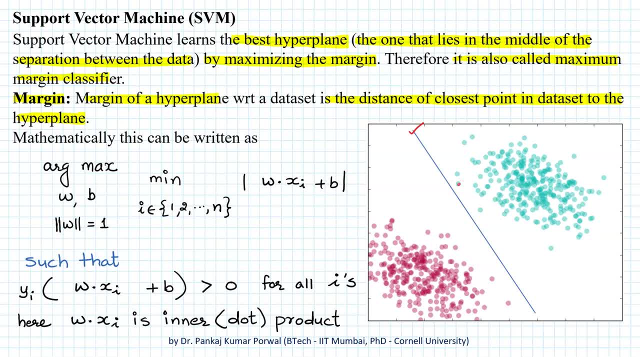 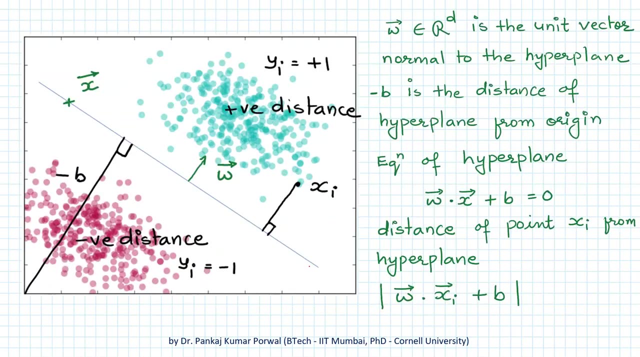 with respect to our data set, then this is the point which is closest to the hyperplane and the distance of this point from the hyperplane will be the margin. And before I get into the mathematics of support vector machine classifier, let us understand some geometrical concepts. Let's say this: 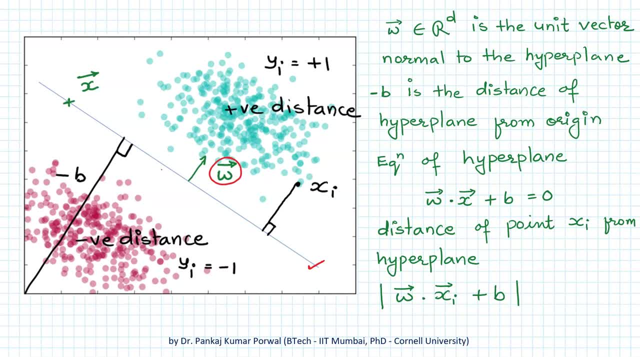 is our hyperplane and w is the unit normal vector to our hyperplane. And if this hyperplane is at a distance minus b from the origin- and here, note, I am saying the distance is minus b and that I will explain in a moment- But if the distance of the hyperplane from 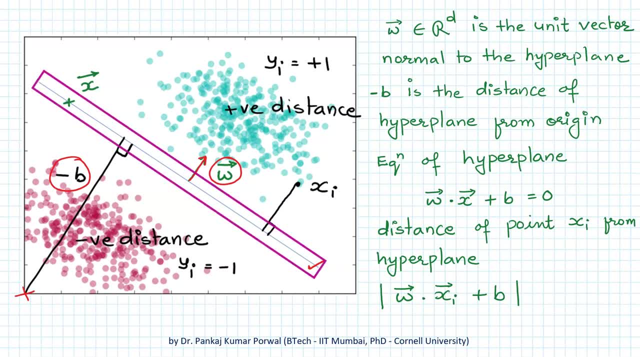 the origin is minus b, then equation of the hyperplane will be of the form w dot X plus b equals to zero, and distance of a point- X, Y- from the hyperplane will be absolute value, wxi plus b. Now, any point which is lying in the side in which the unit normal points will have 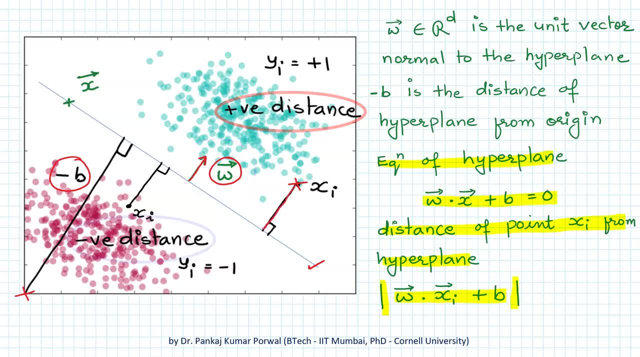 a positive distance to the hyperplane and the points lying on the opposite side will have a negative distance to the hyperplane. So here, when I say the distance of the hyperplane is minus b from the origin, the magnitude of the distance is b and this minus sign shows on which side of 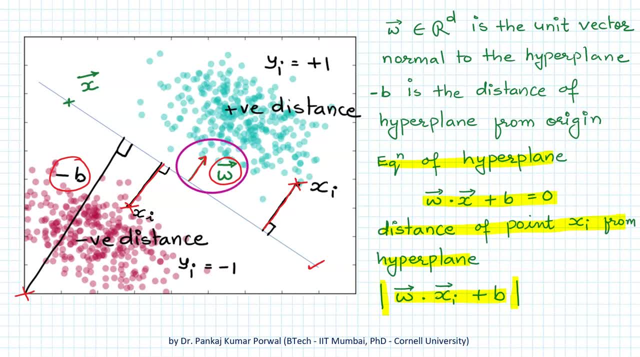 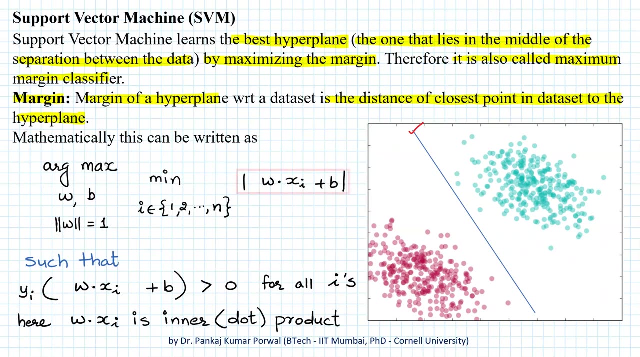 the hyperplane does our origin lie with respect to the direction of unit normal to the plane, And because we always want the distance to be positive, we use the absolute value sign to make the distance positive. So here this expression is the distance of point. 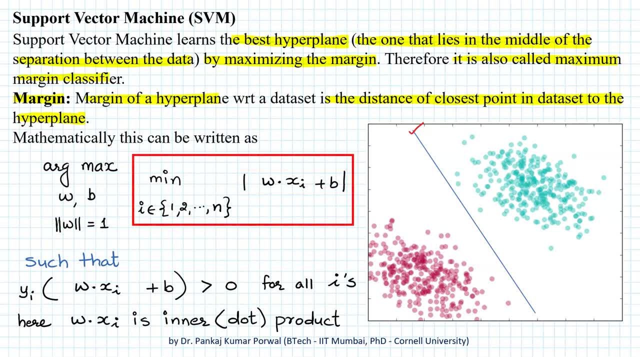 b- This is xi- from the hyperplane and in this expression we are finding the distance for all the points in our data set and choosing the minimum distance, that is, the margin for hyperplane denoted by w and b and the argmax over w and b, with magnitude of w equals to 1. 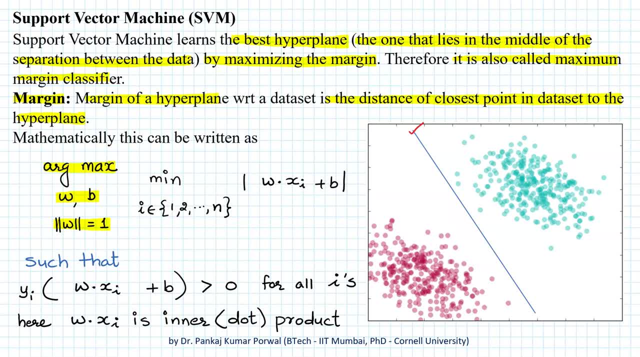 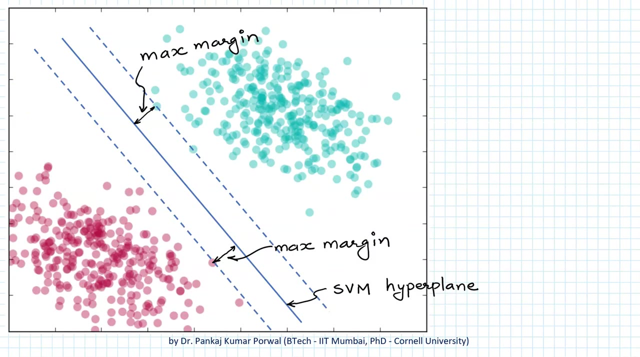 because w is a unit vector, learns the hyperplane. So here we have the margin, for which the margin is maximum, and here this constraint basically ensures that the data is linearly separable. Now there is one thing that people often wonder about, and that is what is the meaning of support vector in support vector machine, So our SVM classifier. 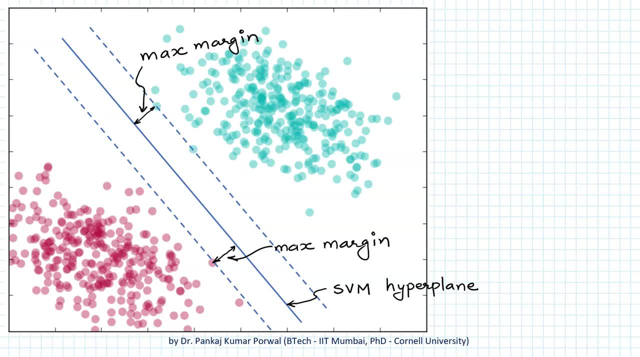 or SVM hyperplane, is obtained by maximizing the margin and there will be points in our data set in both the margin and the margin. So we can see that the margin is maximum and the margin is maximum. So we can see that the margin is maximum and the margin is maximum and the margin is maximum. 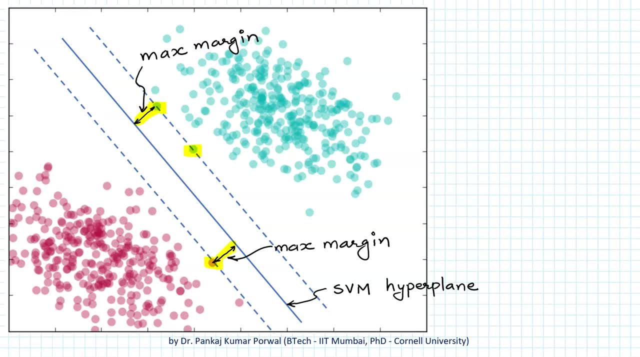 The classes that will be at a distance equals to maximum margin from our SVM classifier. and if these points were not there, then our hyperplane will adjust slightly to maximize the margin. So these points in a way determine the position of the hyperplane. or we can say: these points: 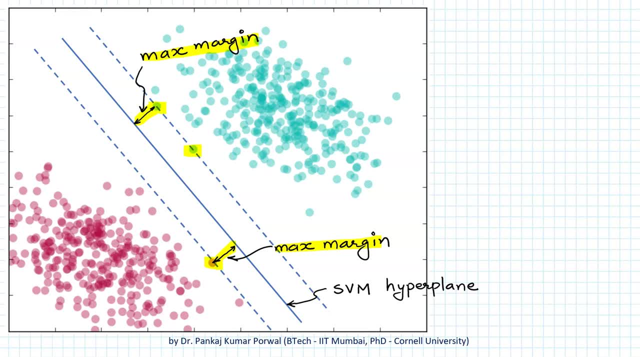 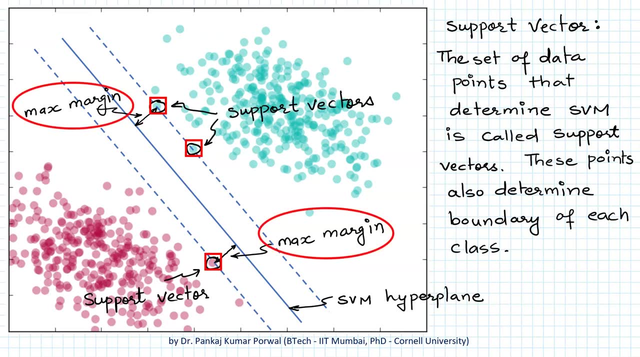 support the hyperplane and prevent it from moving around. So that is why these points, which are at a distance equals to maximum margin from our SVM classifier, are called support vectors, and these points also determine the boundary of each class. That is, all the points of the class lie beyond boundary determined by these points. 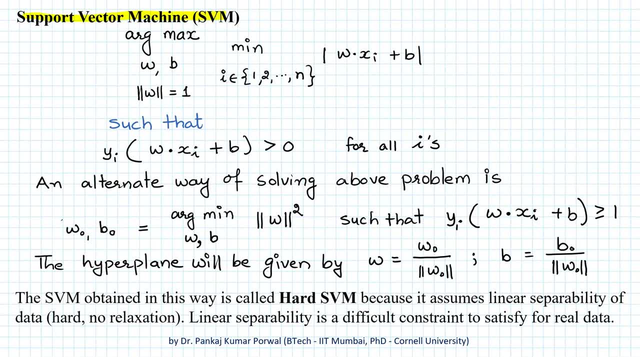 One way of finding support vector machine is to find the value of w and b that maximize the margin, with the constraint yi, w, dot, xi plus b greater than zero. An alternate way of solving the same problem will be to find values of w and b that will minimize. 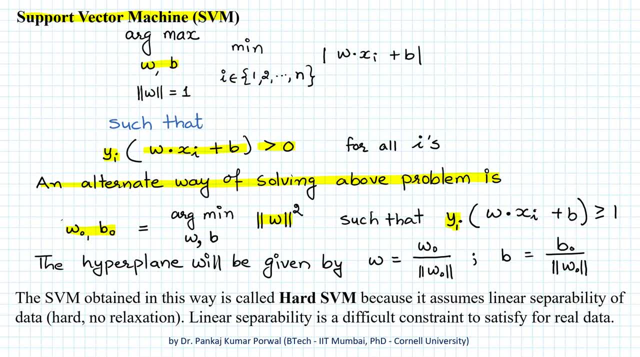 the square of magnitude of normal vector w, with constraint yi into w, dot xi plus b greater than equal to zero. An alternate way of solving the same problem will be to find it with aísimo Psalm thao madri, and it is a doubleθεobar problem. 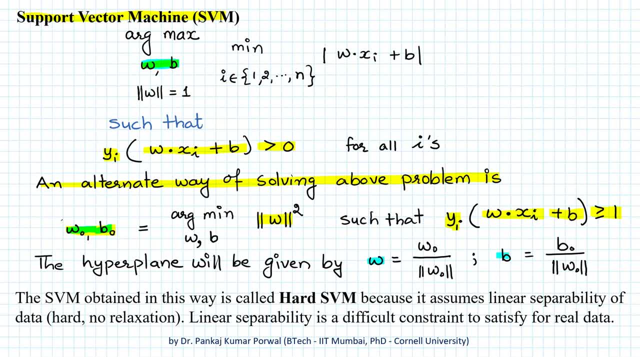 Now let us see how to battling the problem is tries to solve this problem. Just change the environment where your vector zomb is 1 and 0 to b0. in this way, For our result, vector zzi is 0 when vector zzi is 0, while vector zzi is 0 when vector zzi is 0 while vector zzi is 0 when vector zzi is 0. problem is the y and b undetected. For our solution we must get some zar Supreme on boundary vector. Give an exact expression: z and b. modB: 0 walnutM of custom ağ u0 E, b0 to DC. 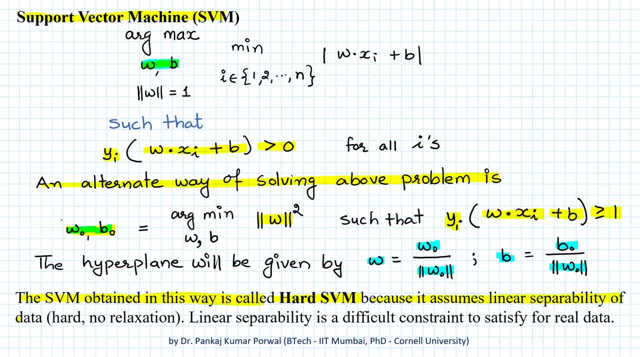 уб mw that the W and B obtain by maximizing the margin. SVM because it assumes linear separability of data, which is a hard condition, that is, one without any relaxation. however, linear separability is a difficult constraint for data to satisfy and to overcome that, we have a softer version of support vector machine.